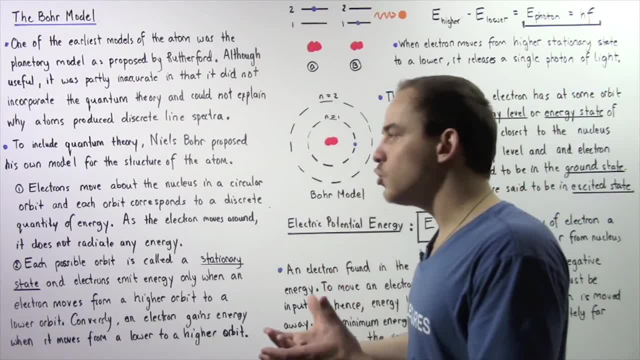 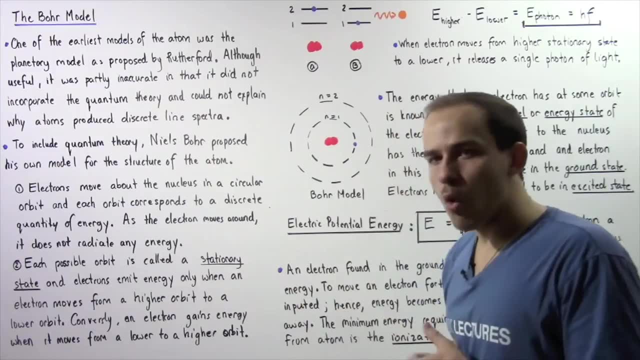 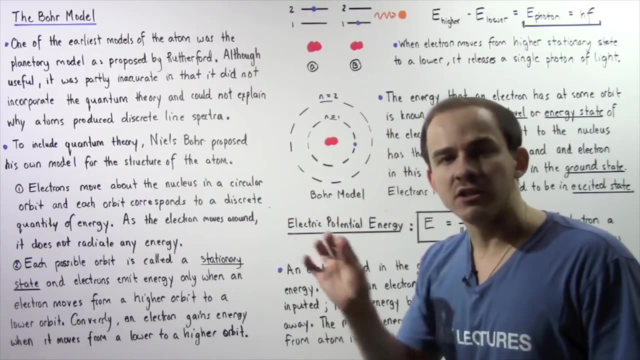 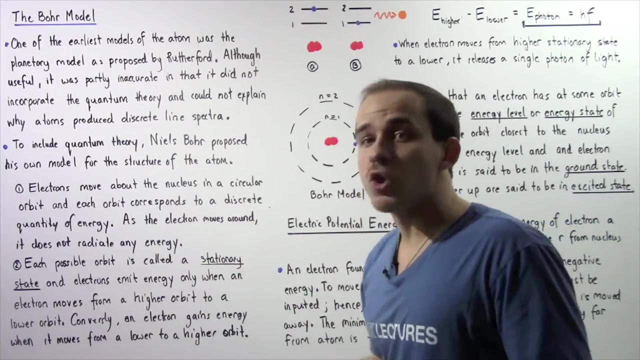 But how exactly does an electron lose or gain energy? That is explained by statement number two. So each possible orbit is called a stationary state and electrons emit energy only when that electron moves from the higher orbit to a lower orbit. And conversely, an electron gains energy. 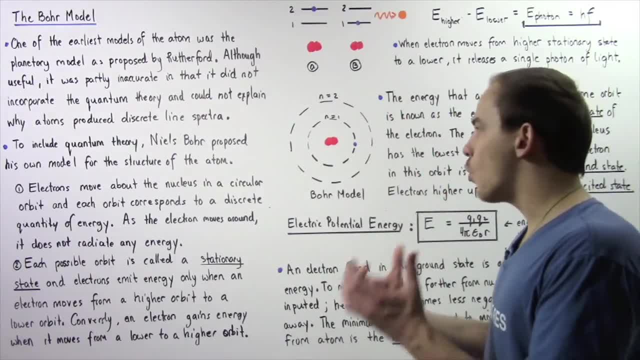 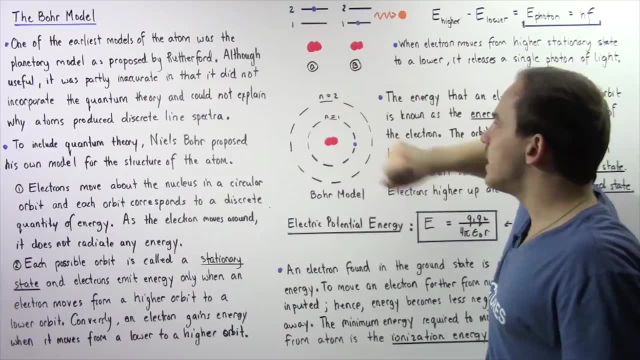 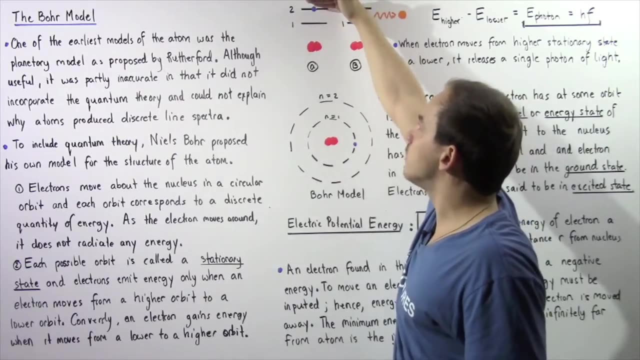 when it moves from a lower orbit to a higher orbit. So let's examine the following diagram. So we have diagram A and diagram B. In diagram A we have the following nucleus, and this is our electron found on the second orbit There's one. 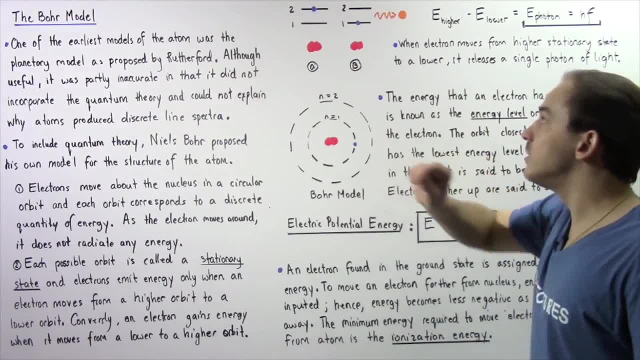 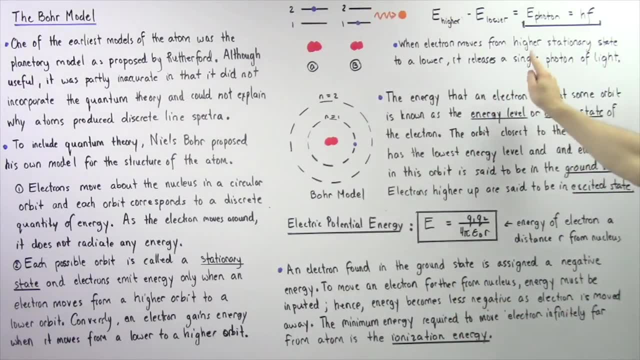 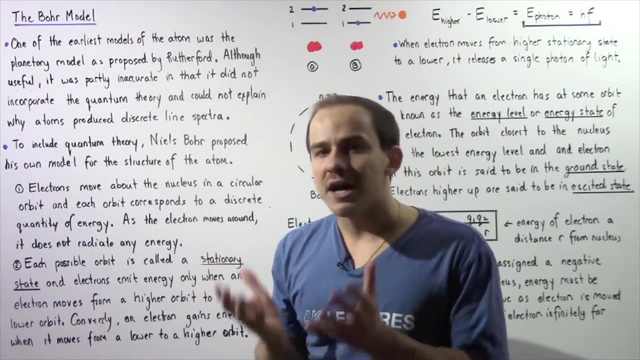 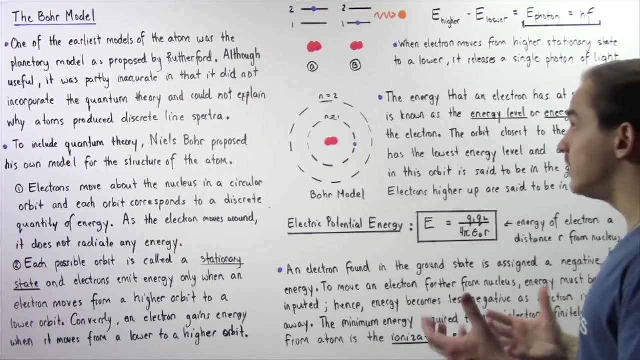 more orbit below that second orbit. So when the electron moves from the second orbit back down to the first orbit, it essentially releases a single photon of light, And that photon of light is a certain discrete quantized amount of energy that is given by the following equation. So to calculate, 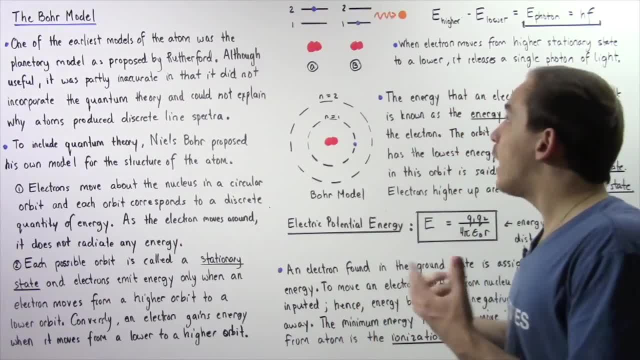 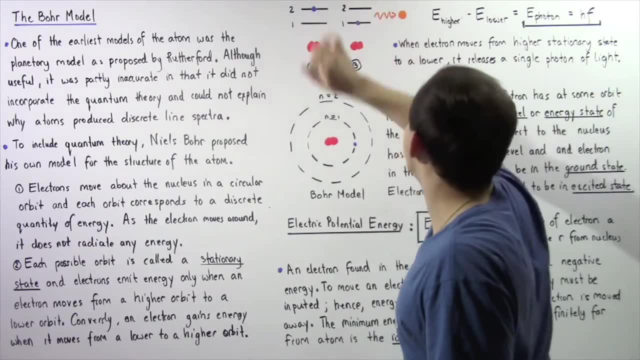 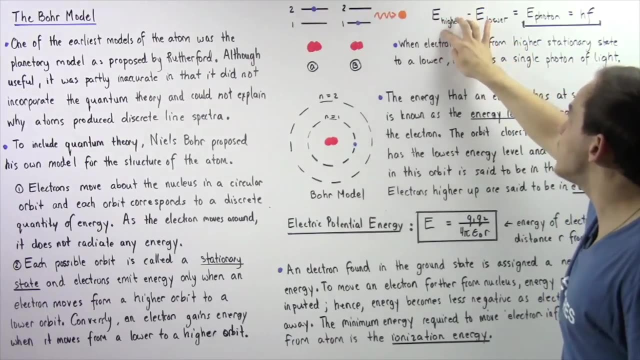 how much energy is essentially released, how much energy the electron loses. we simply take the quantity of energy it had at this point and subtract the quantity of energy it has at this point. So we subtract E higher minus E lower, and that's the quantity of energy it has at this point. 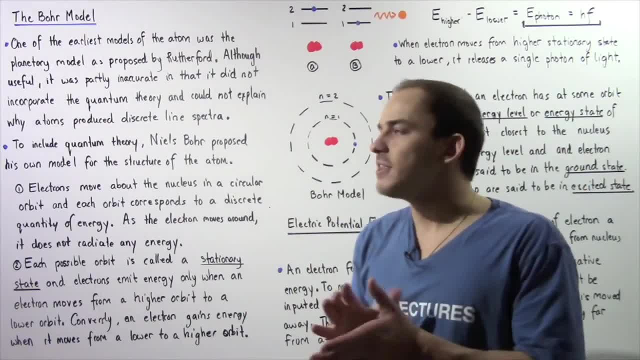 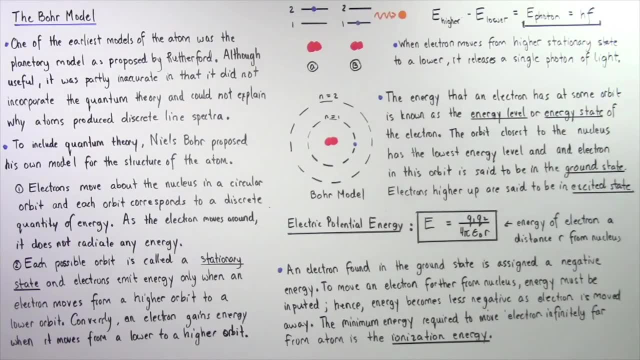 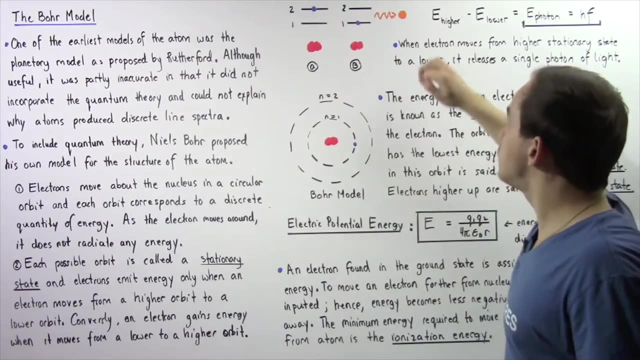 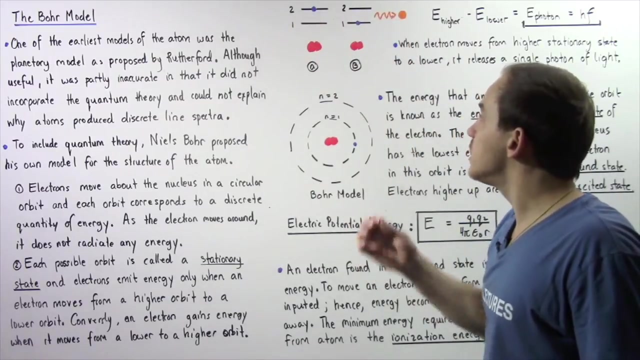 And that gives us the quantity of energy that is carried by that photon, And that is equal to H, Planck's constant, multiplied by F, the frequency of oscillation. So now, conversely, if we examine going backwards, let's suppose the electron moves from orbit 1 back to orbit 2.. To move an electron from 1 to orbit 2,, 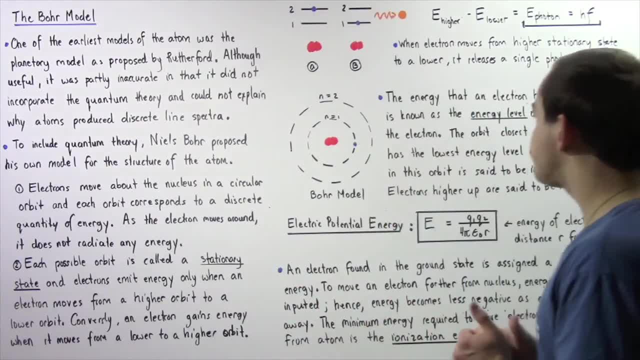 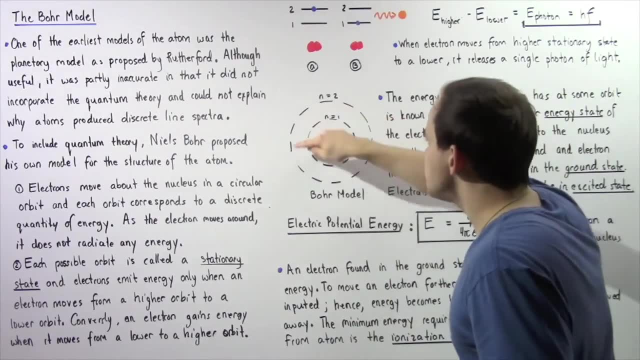 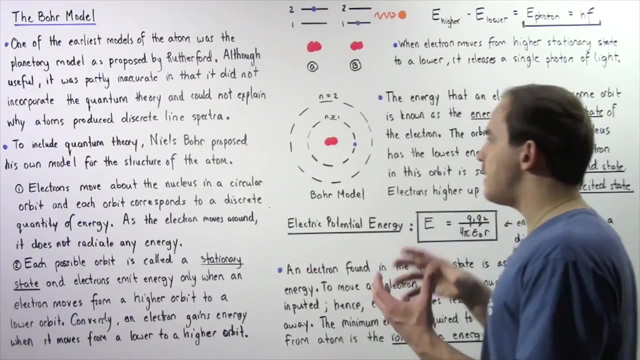 energy must be inputted. So let's look at the following diagram, which basically describes Bohr model. So we have the first orbit, which has N equals 1.. N is known as the principal quantum number. It basically designates which orbit we're referring to. 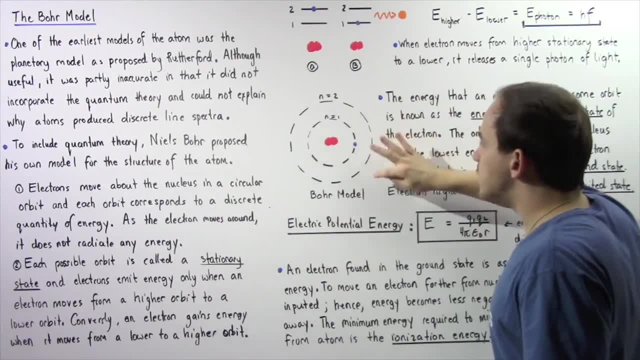 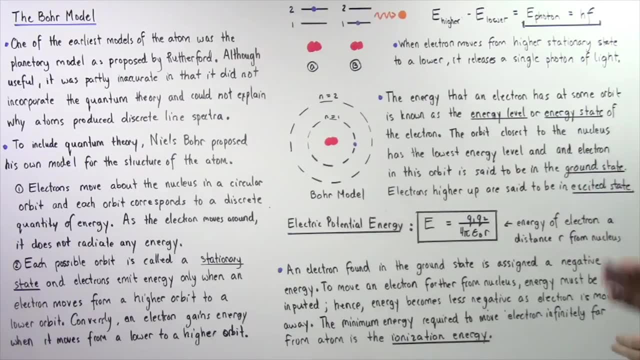 So this electron is found in orbit number 1, but we also have orbit number 2 that is empty for this particular case. Now, the energy that is an electron has at some orbit is known as the energy level or the energy state of that particular electron, or 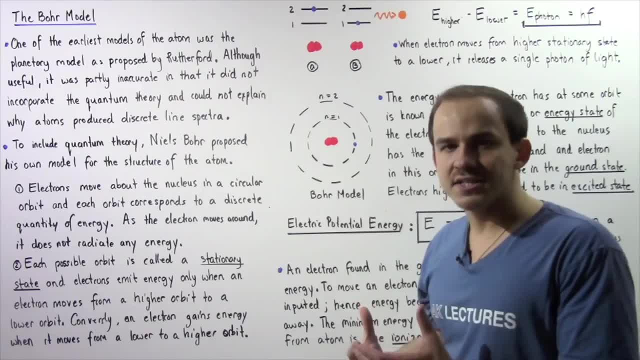 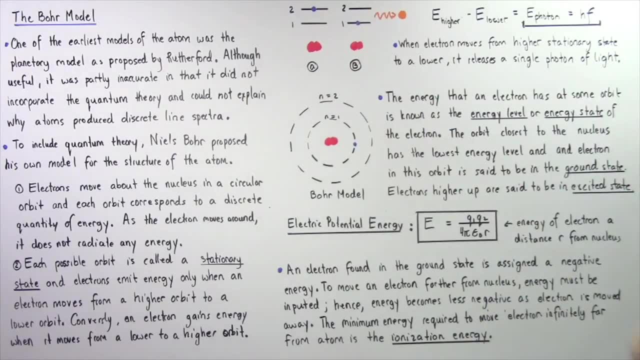 that particular orbit. So not only is energy quantizized but orbit are also quantizized as involved by these positive integers. Now, the orbit closest to the nucleus has the lowest quantity of energy. but orbits are also quantizized as shown by these positive integers, The orbit closest to the nucleus has the lowest quantity of energy. so each one has a say or size, number or magnitude. So based on here, orders, Кол and Qs. 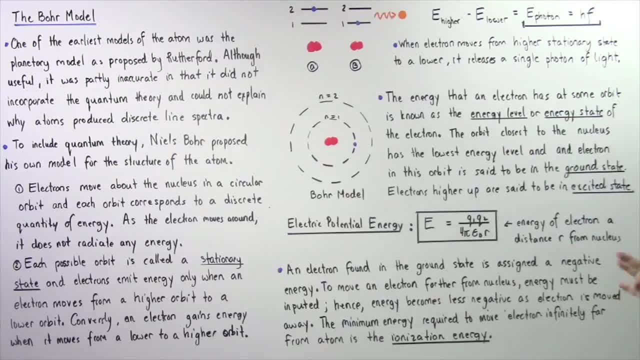 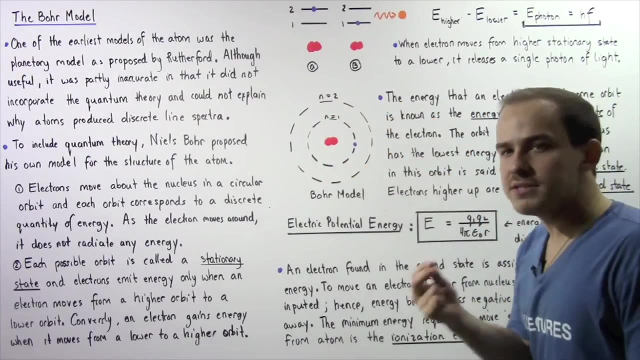 has the lowest quantity of energy level and the electron in this orbit has the lowest quantity of energy and is said to be in the ground state. So for this particular case, this orbit corresponds to the ground state of our electron. If the electron is found in this orbit, that is lowest. 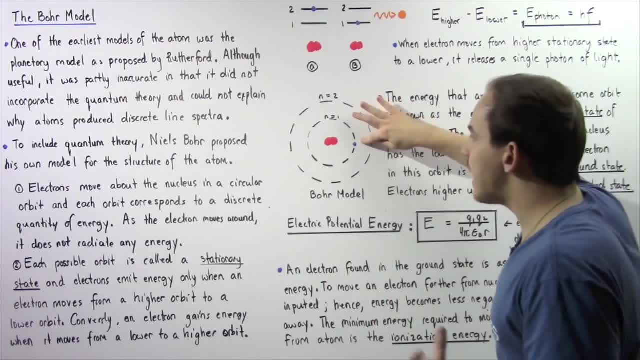 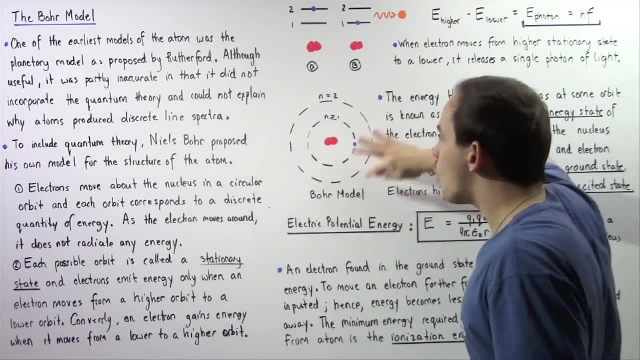 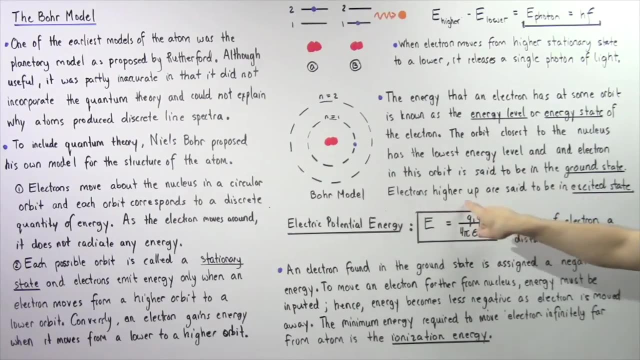 in energy and closest to our nucleus, the electron is said to be in the ground state. However, if we take the electron and move it to the second orbital, the electron is now said to be in the excited state. So electrons higher up with respect to the ground state are said to be in the excited. 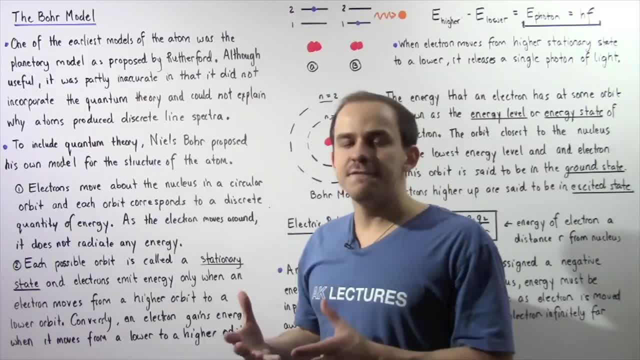 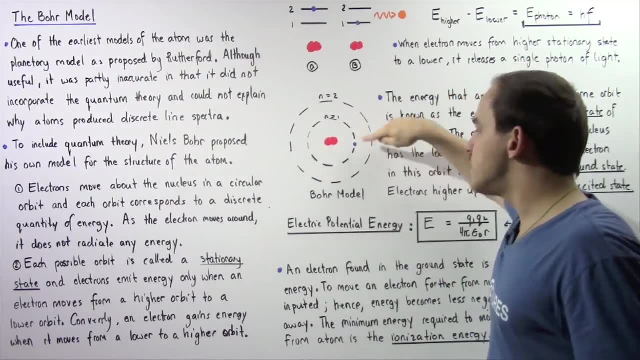 state. Now, how exactly do we define the energy of the electron relative to energy? Well, we can define the energy of the electron relative to the excited state, It's position with respect to this nucleus. So we discuss the electric potential, energy because 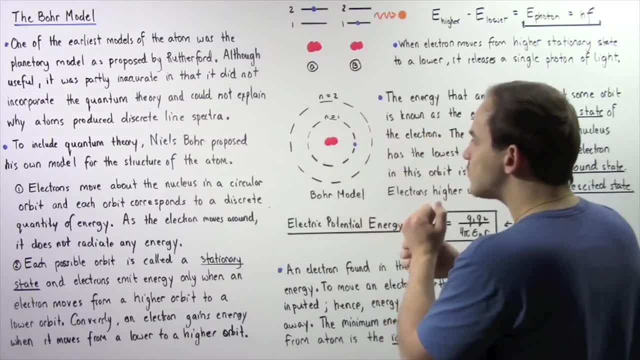 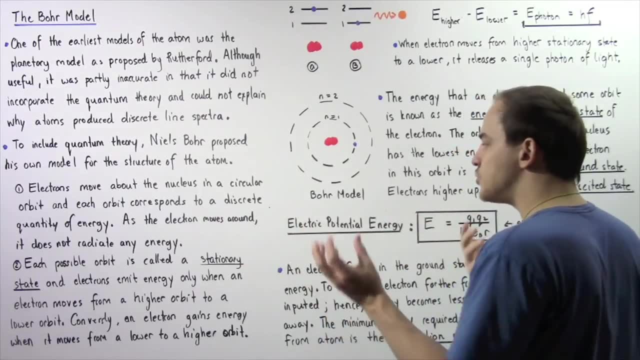 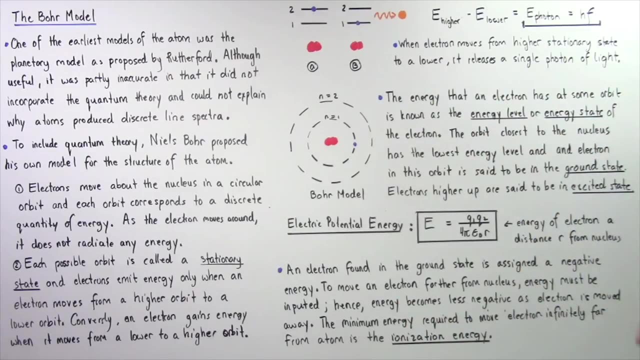 we're dealing with a negatively charged electron and a positively charged nucleus, So we essentially have a separation of opposite charge, And that means this electron will have a certain quantity of electric potential energy. that is given by the following equation: So the electric potential energy E is equal to Q1, the charge on the electron multiplied by Q2,. 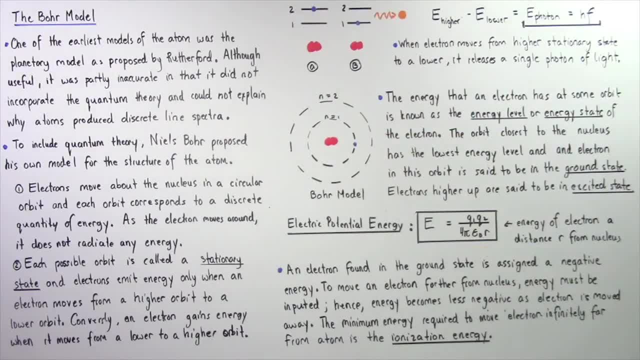 the charge on the nucleus divided by 4 pi, epsilon naught- multiplied by R, where R is simply the separation distance between the electron and our nucleus. So this equation gives us the energy of the electron a certain distance, R, from the nucleus. Now 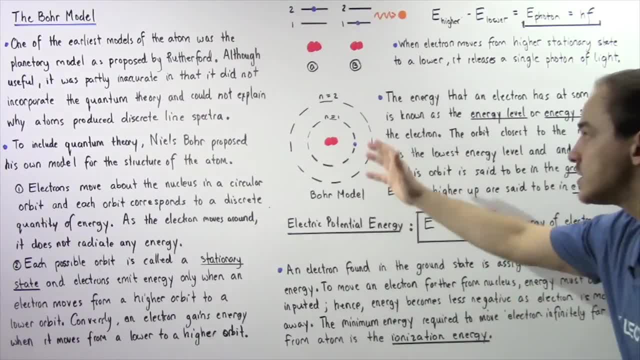 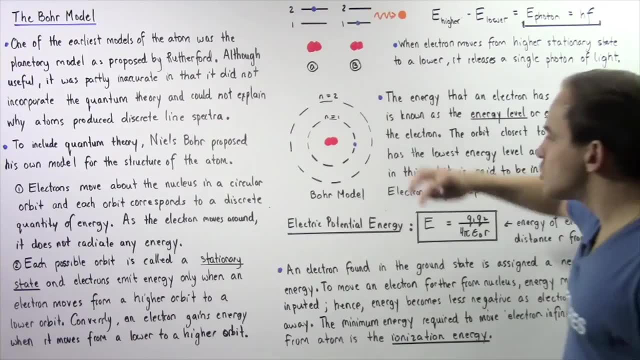 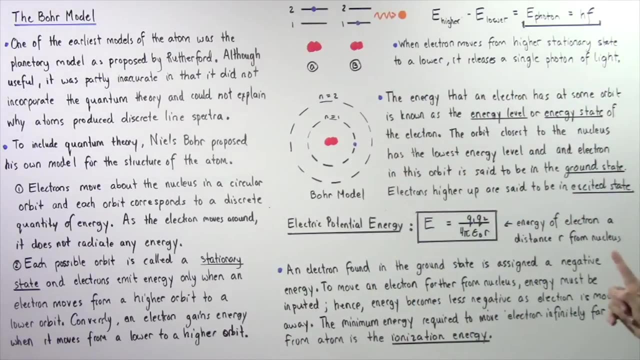 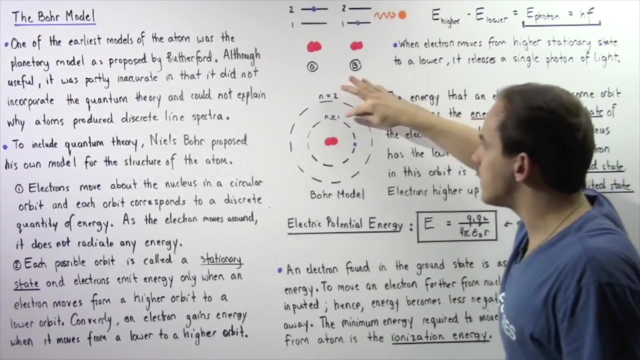 relative to the energy of the electron drag on the electron, which they've written previously. if we were to absorb the energy in the an electron with the amount of current in it, then if we made this little equation in judge this, So we got that function in contrast. So 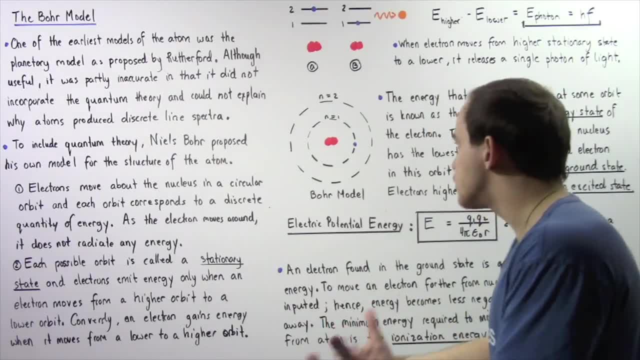 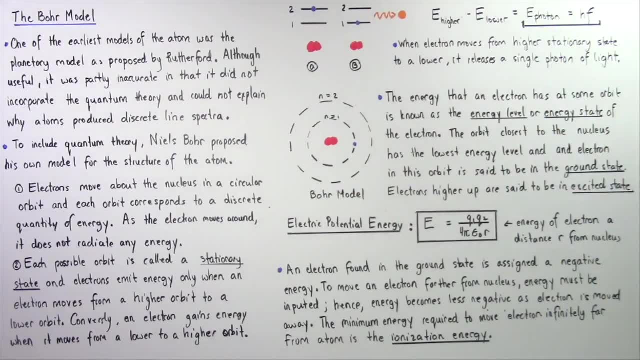 to this discussion. energy must be inputted, So that means the energy becomes less negative as we go farther away from our nucleus. So once again, to move an electron farther from the nucleus, work must be done on that electron, and so energy must be inputted. Therefore energy becomes less. 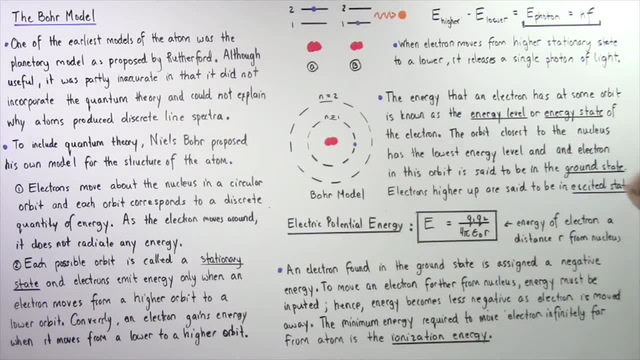 negative as the electron is moved farther away from that nucleus. Now we define ionization energy of our electron in the ground state as the minimum energy that is required to move an electron infinitely far away from the ground state, from that atom. So notice if we look at the following: 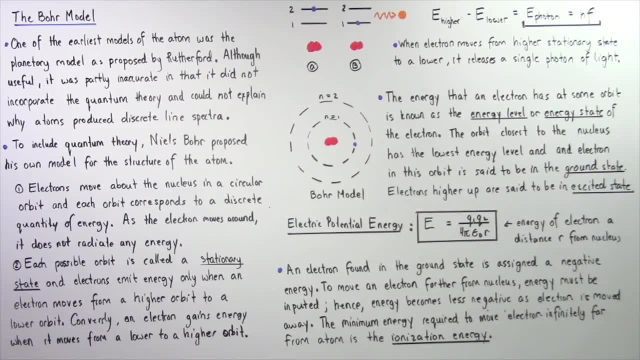 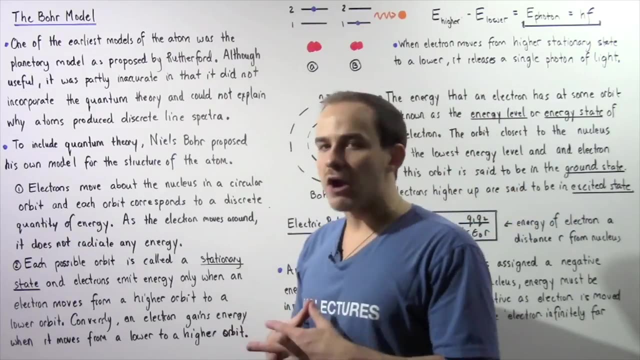 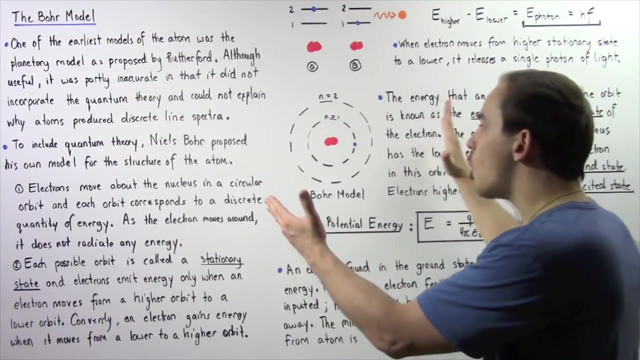 equation: when r is infinitely large, meaning when the electron and the protons in the nucleus are infinitely far away, the energy of our electron will be zero. So we define the electric potential energy of our electron when it's infinitely far away to be zero And when the electron moves closer to our nucleus. 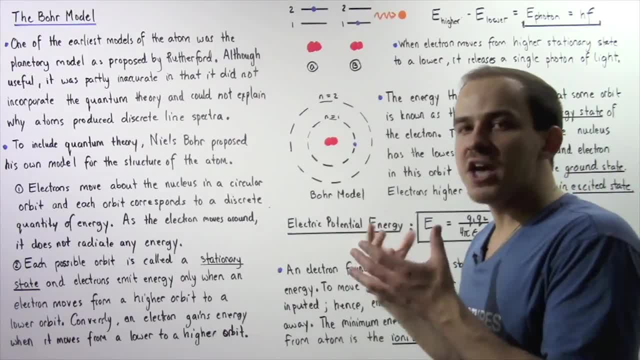 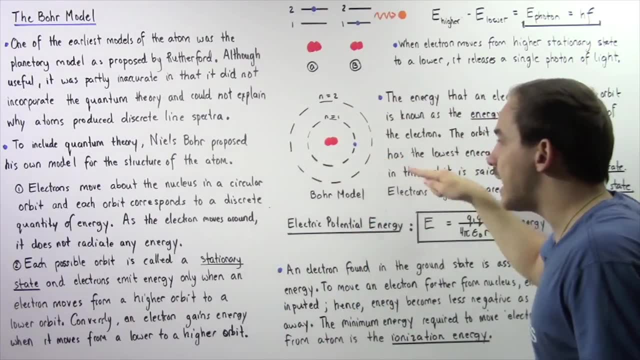 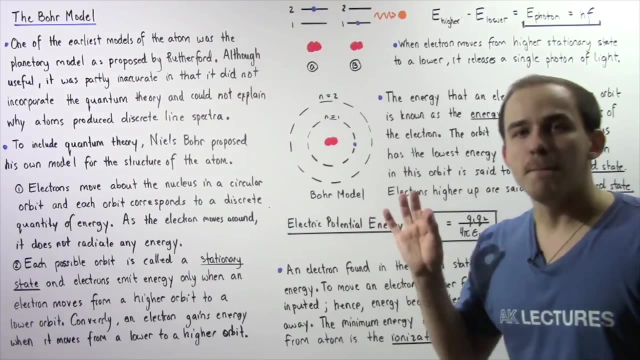 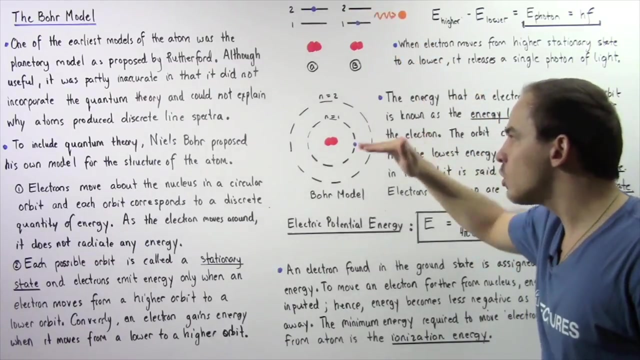 it essentially lowers its energy. the energy becomes more negative And when the electron is found in the ground state, that represents a position where the electric potential energy of the electron is most negative. So, once again, as electron moves from a higher orbital to a lower orbital, it decreases in energy, meaning the energy becomes more negative.